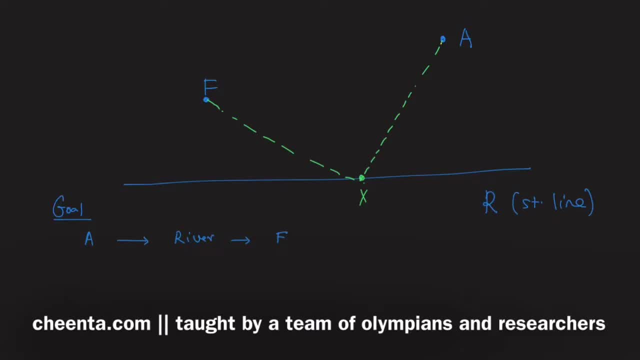 Or you could choose some other point. maybe. Maybe you can go straight from the point A to the river and then from that point to F. So there are many paths. There are many paths from A to the river and from the river to F. 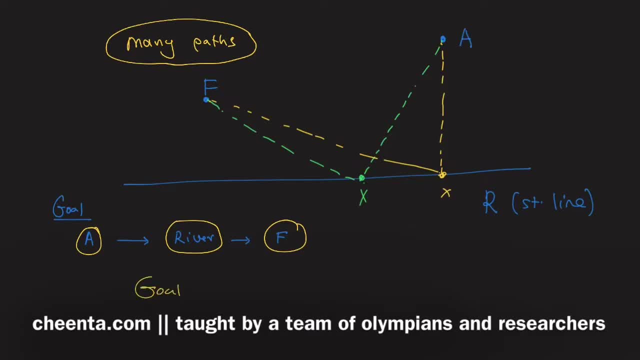 Our goal is to find the shortest path. Find the shortest path from A to the river, to the friend's house, So you can pause the video here and give it a try, Because this is a problem of a geometric transformation called reflection, And that's what we are going to learn in this particular video. 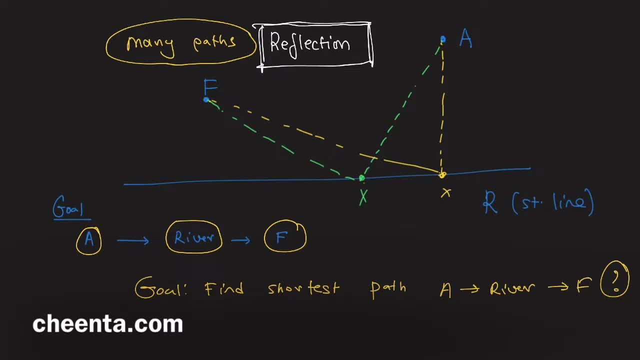 Reflection is a very powerful geometric transformation. Many difficult geometry problems can be easily solved if you know how to reflect. It's an isometry, which means it preserves the size. In fact it's called size. There is a precise meaning of the word isometry. 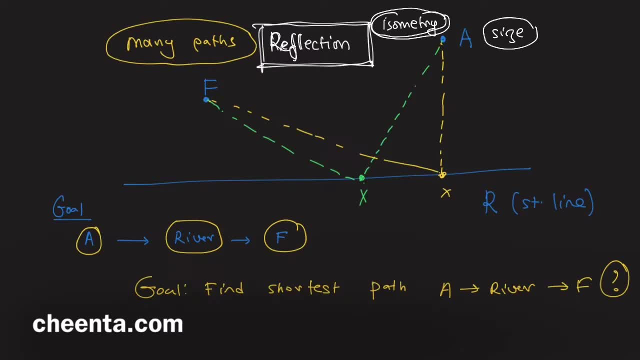 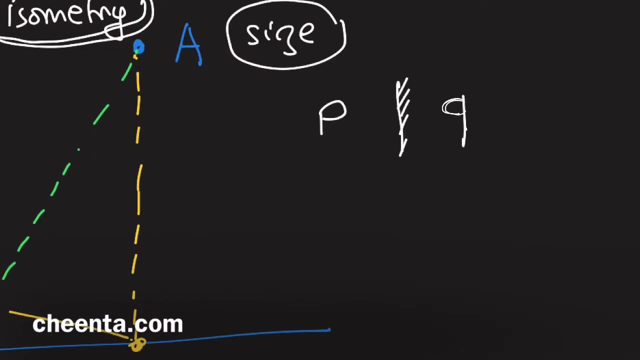 But for the moment, if we have the letter P and if we reflect it about a mirror, then the output, that is, the reflected image, will have the same size. A more precise meaning of isometry is this: that if you take any two points on P and if you take the image of those two points, 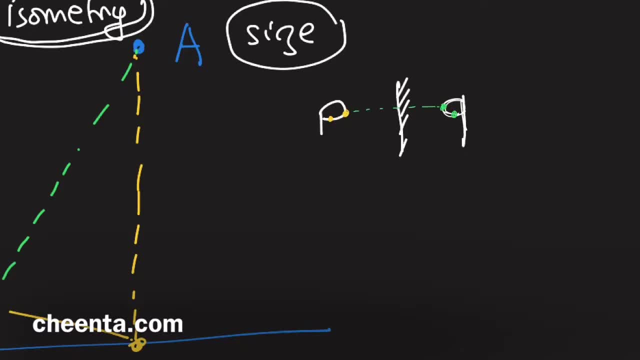 so image of this point is point A is A prime, image of B is B prime. then the distance between A- B and distance between A prime, B prime will be same. So that means isometry is a geometric transformation such that the distance between point 1 and point 2 and their images. 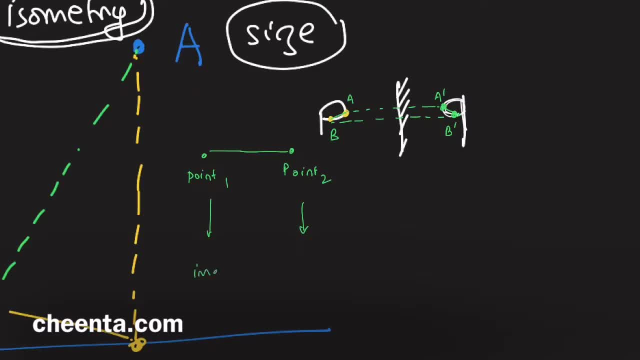 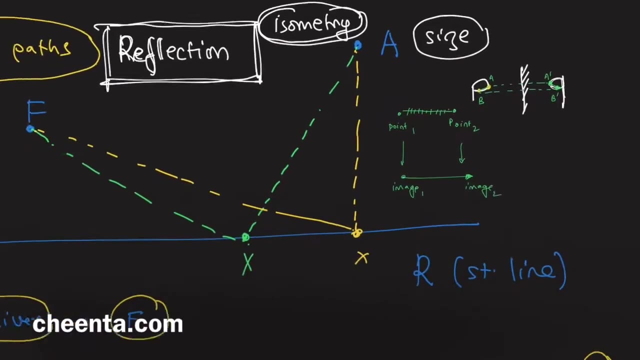 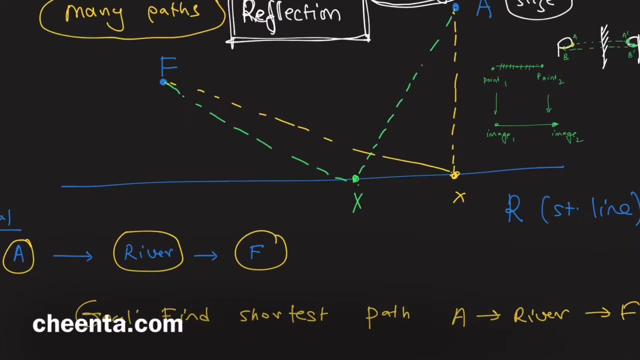 whatever the initial distance was, the distance between image 1 and image 2 will be the same. So isometry preserves the distance between any pair of points. However, this reflection does not preserve orientation. Anyway, how can you find the shortest path from A to the river, to F? 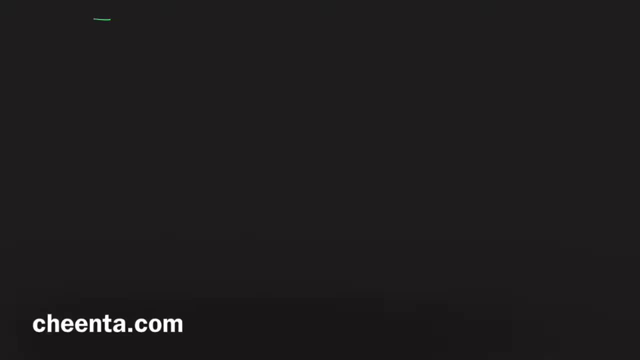 This is how you can think about it. This is also a problem of triangular inequality, And in its simplest form, triangular inequality says that if you have two points, A and B- then the distance between A- B- there is a segment A- B- is shorter than if you take any other point. 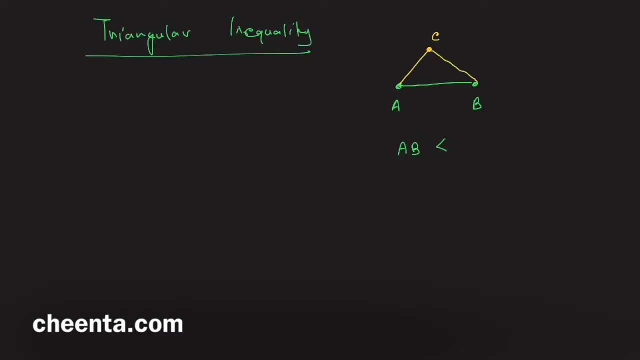 And go from A to that point and then to C. So it's less than AC plus BC. So this is really the definition of a straight line. So triangular inequality is in disguise the definition of a straight line. It says that the shortest way to go from A to B is the segment joining AB. 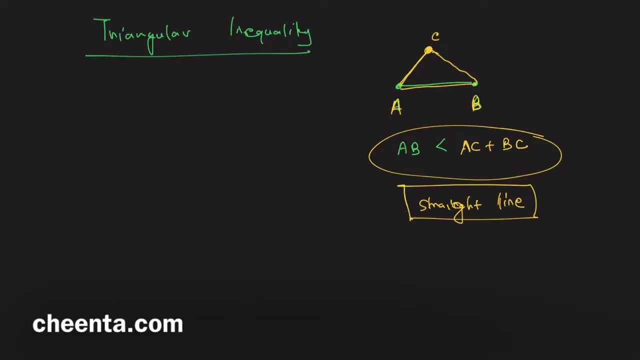 If you take a roundabout turn via some other point C, this will be larger. okay, Alright, so let's come back to our setup. We have the river L R, the point A and the friend's home at F. 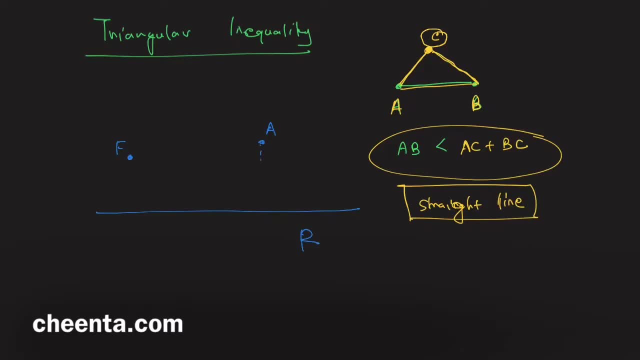 So the solution is something like this: You reflect A about the river, So you have to think of the river as the mirror. This is A' suppose. Now join A' F. Join A' F Wherever A' F intersects the river. that is our desired point X. 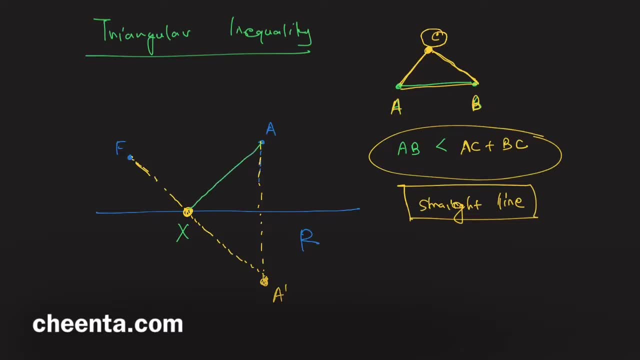 So let's join AX now. This path, that is, AXX, F, A to X, X to F, This path is the shortest. Now why is that? If you pick any other point Y, let's pick this point Y.